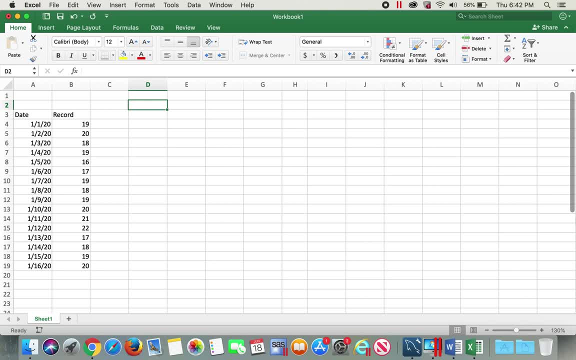 Today I'm gonna show you how to create upper control limit and lower control limit control chart. Usually this UCL and LCL control chart is used in, or the control chart in general is used in statistical process control, kind of like in a quality control areas in production etc. here I have date values. 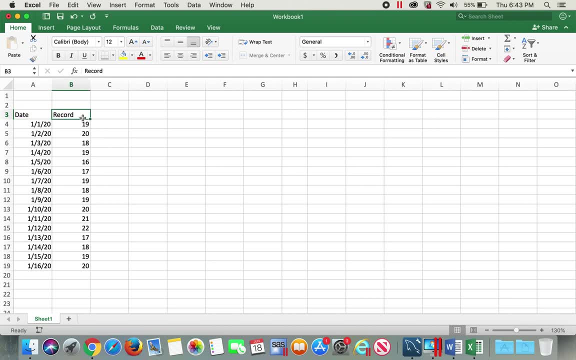 18 date values and records, or measurements, however you want to say it. I have 18 records too. In order for me to create statistical process control chart with upper control limit and lower control limit, I'll have to first find out mean and standard deviation of these records. for that, what I'll do is I'll 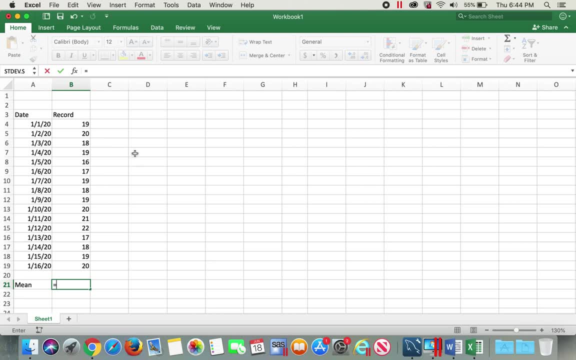 type in mean and then equals to for mean, I'll type in average average open braces and I'll highlight all of these and then I'll close braces. enter: here's my mean value over here. so what I'm gonna do is I'll copy this mean value to the table or i'll just go ahead and type it in 18.875 and if you double click this, 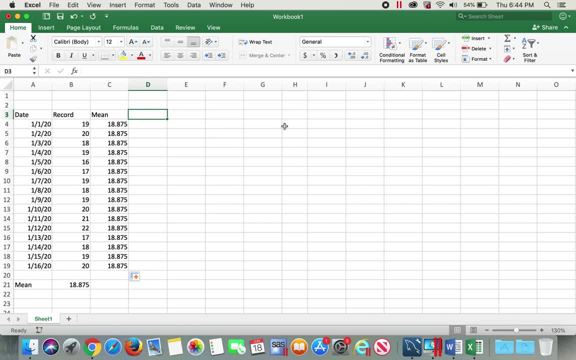 it will automatically auto populate the whole table. now the second part is to calculate the upper control limit, um. the upper control limit formula is mean plus three standard deviation. so ucl is going to be equals to mean value, which is this, and then plus three times three, multiplied by standard deviation sample, which is s instead of population. 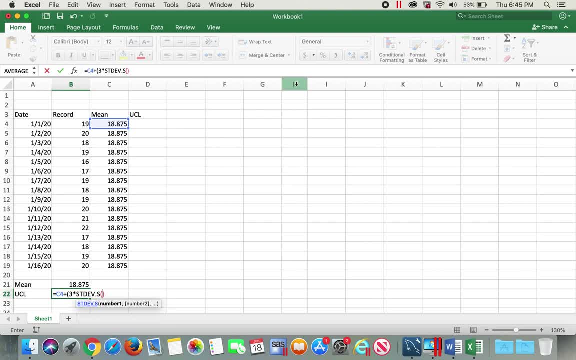 since we have only 18 records and standard deviation will be, will highlight all of these values, records and then close braces, enter and here's my standard deviation or ucl value. so what i'm going to do is i'll type in this value here: 23.506, 4145- same thing like previously, i'll double click it and it auto fills it. 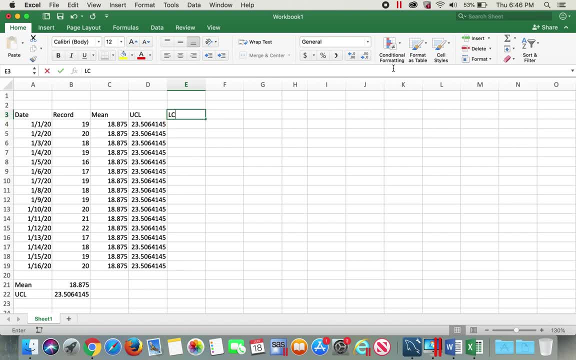 now the third part is to calculate lcl, lower control limit. uh, the formula for lcl is mean minus three, standard deviation equals two. our mean is here minus three multiplied by standard sample standard deviation of these values. and then close braces again enter. here's my. 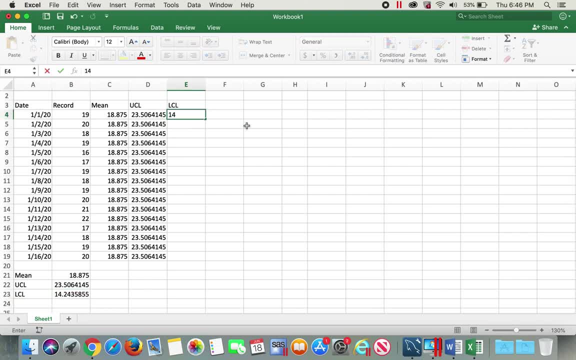 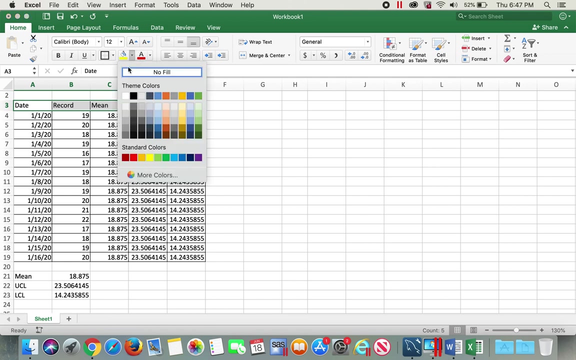 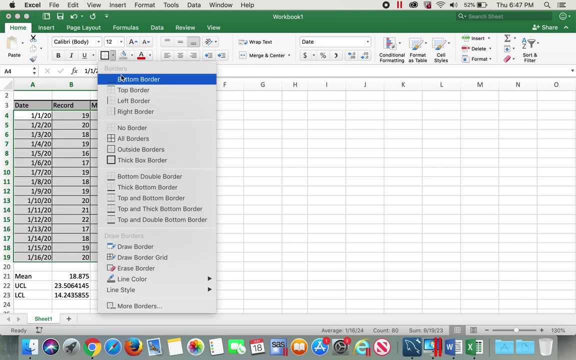 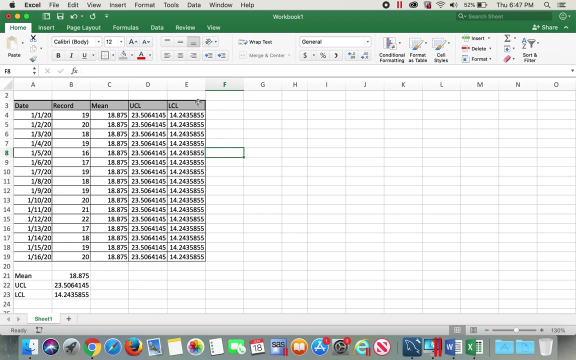 lcl value. i'll go ahead and type in my lcl value to 14.24, 35855 and double click this to auto fill it. so now we have all the required data. i'm going to just make a nice table here now. what i'm going to do is 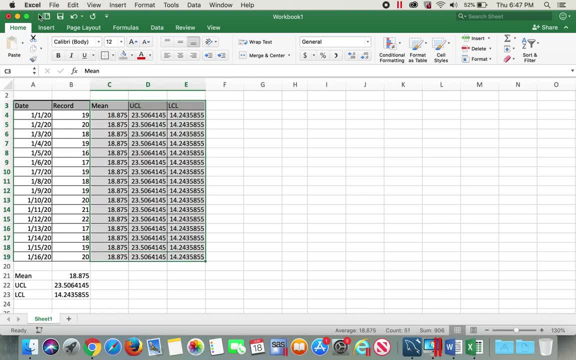 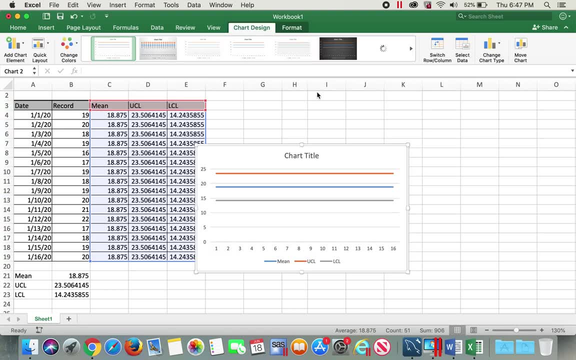 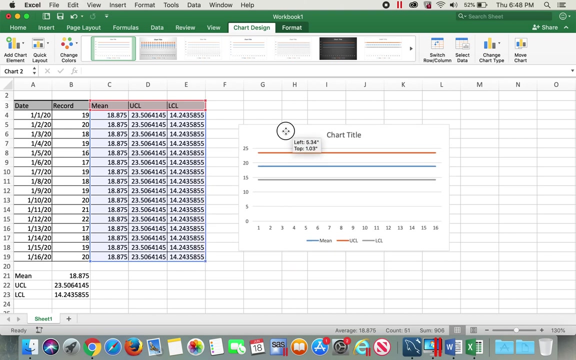 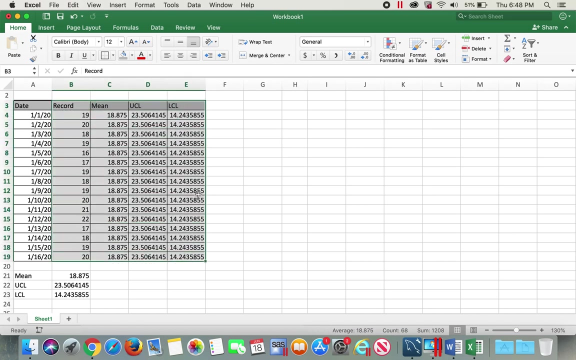 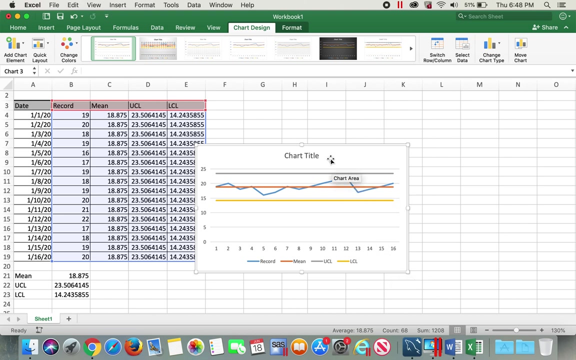 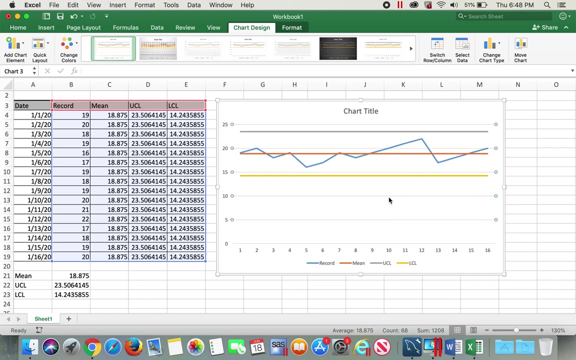 select all three of these values and then insert a chart. here i'll choose my chart and here is our mean. what i'm gonna do is delete this. i actually will have to select all four of these values and then choose the chart, and here you go. this is the chart that we're looking for. i'll delete these. i'll put chart title as: 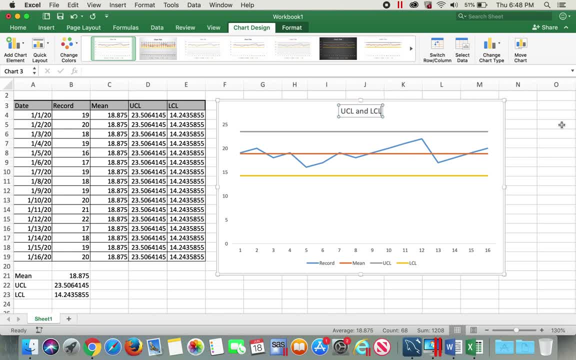 ucl and lcl control chart um. in order to put the label, i'll click in the last value and then right click it- add data label and i'll type in: complete this type in ucl. i'll go ahead and move this over here and then for this. 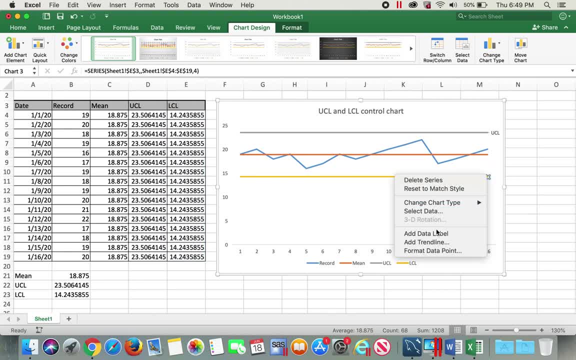 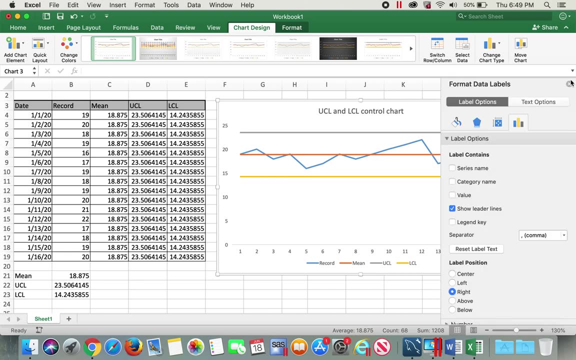 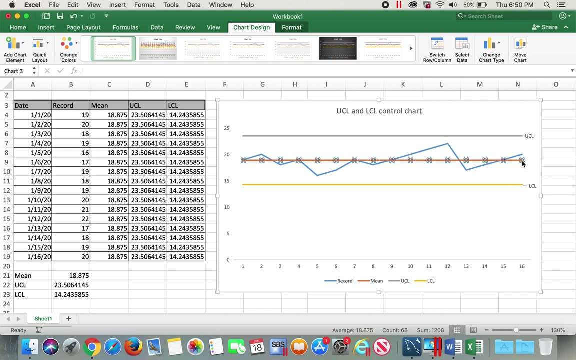 This one same thing. right click it, add data label, Delete this type in LCL. There you go. now I'll do this again and this is our mean value: data label, mean and this is our record.